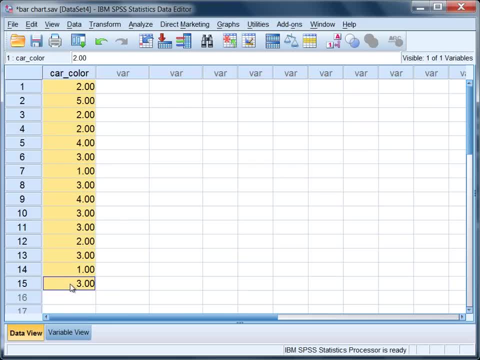 And what I've done in this example is I've already entered my value labels. So, for example, if I click on this button right up here, then I'll see the colors that the different numbers correspond to. So notice, we have 1,, 2,, 3, 4, white cars were observed, and so forth. I'm going to turn these off for now, but you'll see how they're very useful in just a moment when we produce our bar graph. 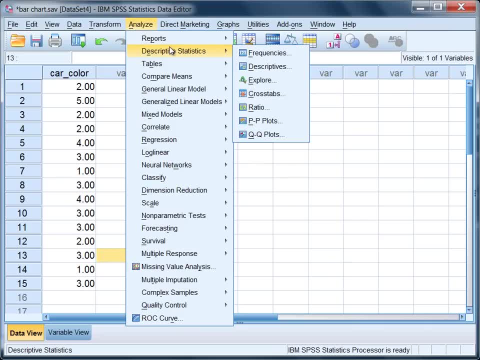 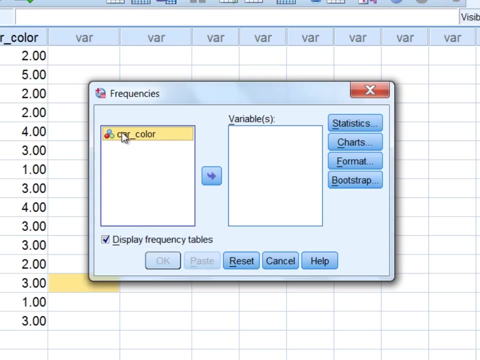 To produce a bar graph. let's go to Analyze and then Descriptive Statistics, And we can actually use the Frequencies command to produce a bar graph And then we can also use the graphs. I'll show you both ways. So we'll start with this: Analyze, Descriptive Statistics, Frequencies, And then here I'm going to. you should see your window look like this. I'm going to move carColor over to the Variables box, select Charts. 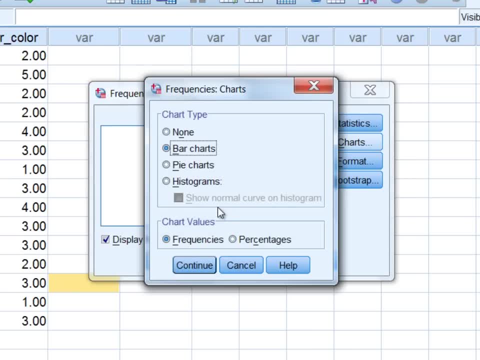 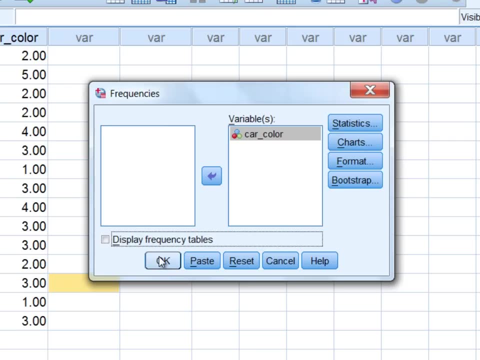 And then here I'm going to. you should see your window look like this. I'm going to move carColor over to the Variables box, select Charts. And then here we want to select a bar chart, Click Continue. Let's deselect the Display Frequency Tables and then click OK. 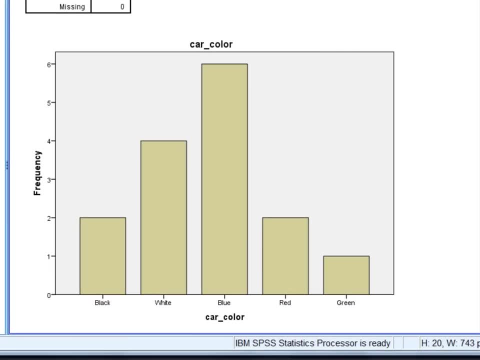 And notice here. in this case we get a bar chart where the variable is CarColor on the x-axis, The frequency is on the y-axis And we have our different car colors here And the height of the bar indicates the frequency. 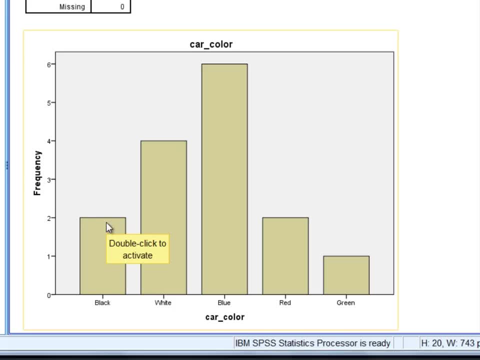 the frequency or how many of each color car was observed. So we have: two black cars were observed, four white cars, six blue cars, two red cars and one green car. Now, many of the options on this chart can be modified and I'll show you one quick modification we can make. If I double click on this chart, what will happen is that: